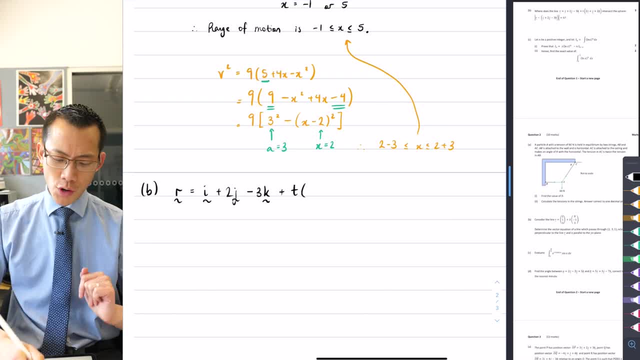 it doesn't matter, the parameter can be called anything. And then you've got 2I plus J plus 2K. There's our straight line. Our sphere is going to be R. take away, and then this should look suspiciously familiar to you: 2J minus 3K. You can see, in fact. 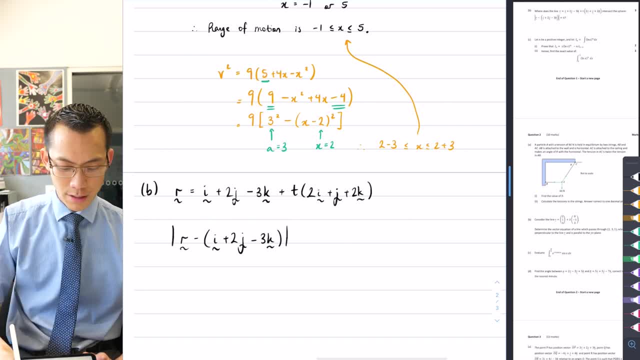 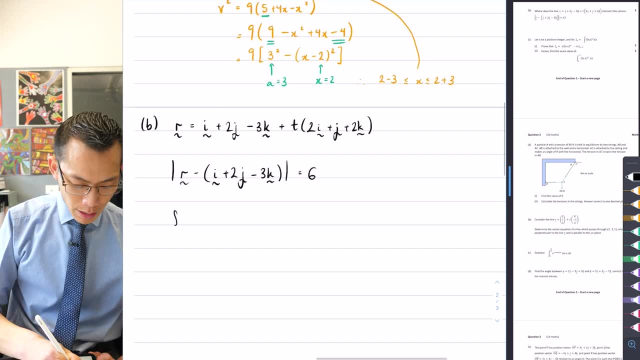 that matches the vector that you got up here, that positions the line, And what's that going to be equal to Six. So there's our radius, of our sphere. So solving simultaneously. as promised, what I'm going to do is I'm going to substitute the line into the sphere equation. that looks like: 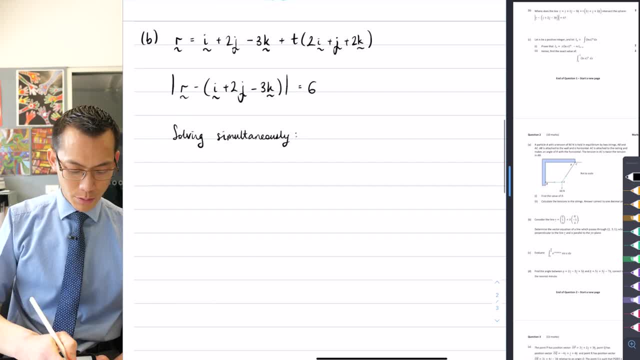 the most straightforward way to do it, So solving simultaneously, I'm going to substitute all of this R- yeah, I'll just stay with orange, that's fine. All of this R into this R, right here. Okay, so therefore I get I plus 2J minus 3K. plus, here comes the parameter T: 2I plus J. 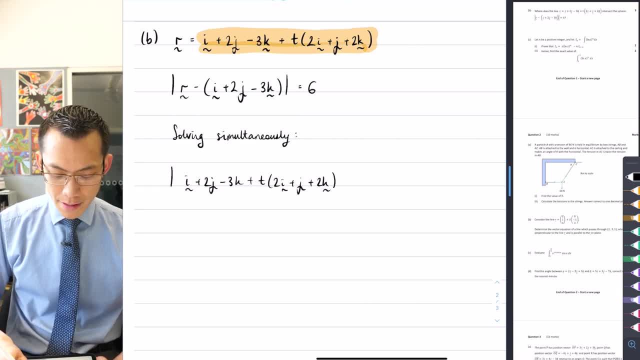 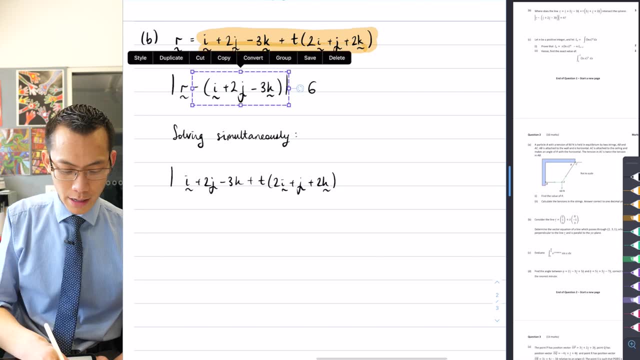 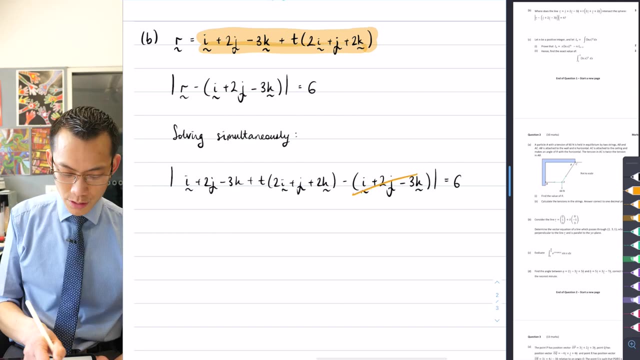 plus 2K. And then there's the substitution into R, And what I subtract is this same vector that I had here. So I'm going to subtract that and close off my absolute value. That equals to six. So you can see here this is going to cancel with all of this, so that 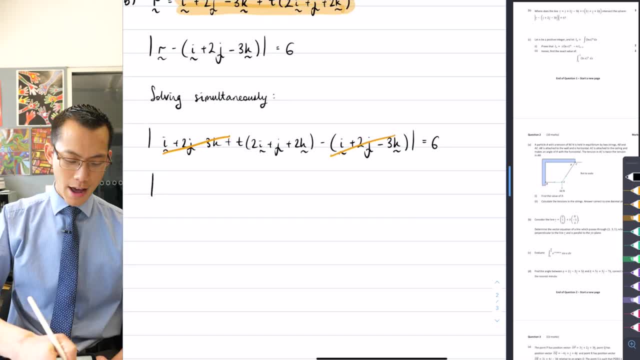 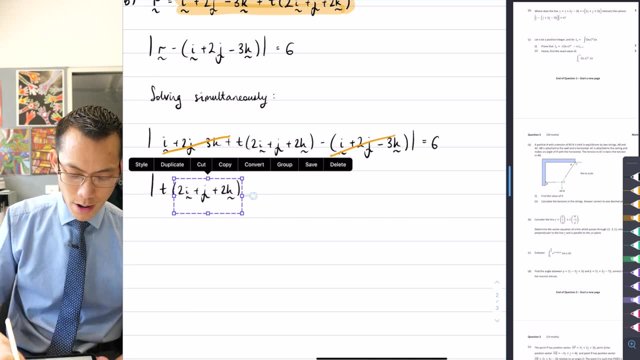 gives me the absolute value, starts again. You get that T in there and then you've got- in fact, I don't know what you've, why I wrote that separately- all of this comes along for the right close that and that equals to 6.. Alright, now, this is the part. I then need to go. 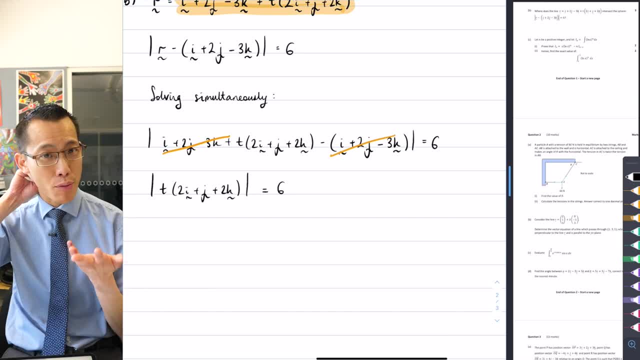 and solve. I'm really looking for the values of the parameter, like. particular values of the parameter will get you onto particular points on the line, So there are going to be, I expect, a couple of different places that the line will intersect with the sphere. I'm just assuming that. 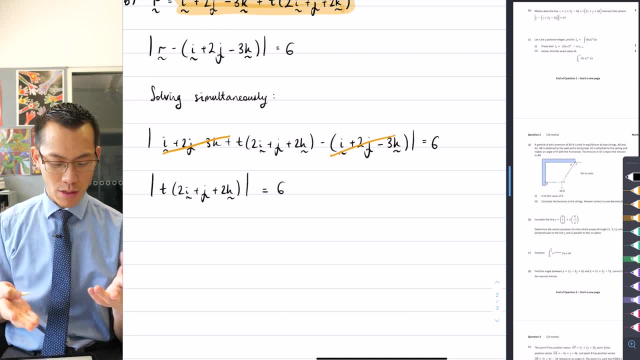 it's a secant. I may well find that there are no points of intersection, so there will be no solution for t. or it is possible that this line is tangent to the sphere, which would mean that there is a single value of t that actually works. So let's try and solve this and see what emerges. 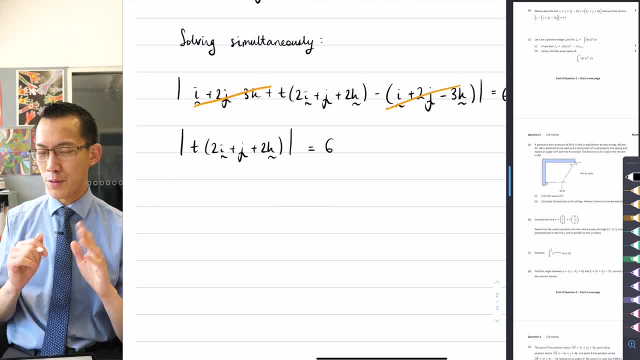 I can get rid of all of this absolute value notation, or the absolute value notation that is relevant to get rid of, by saying: let's pull out the parameter there, t, and then apply that absolute value to this, which is what's the distance to the point at the end of this position. 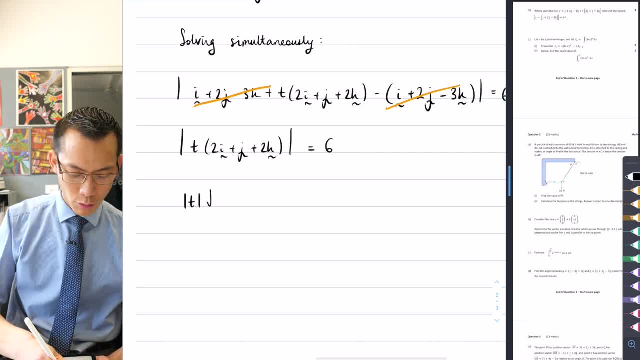 vector. So this is just Pythagoras. yeah, It's going to be a point at the end of this position vector. so this is just Pythagoras and this is going to be the square root of 2 squared plus 1 squared plus 2 squared. I'm just 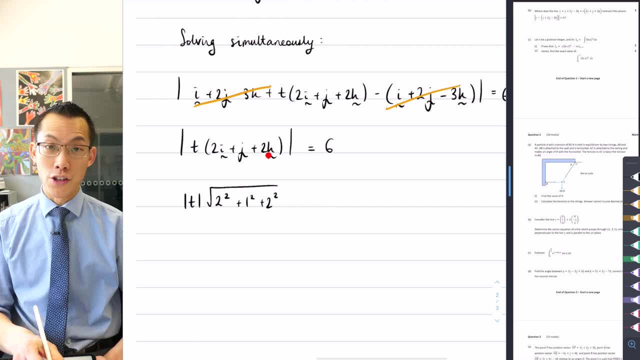 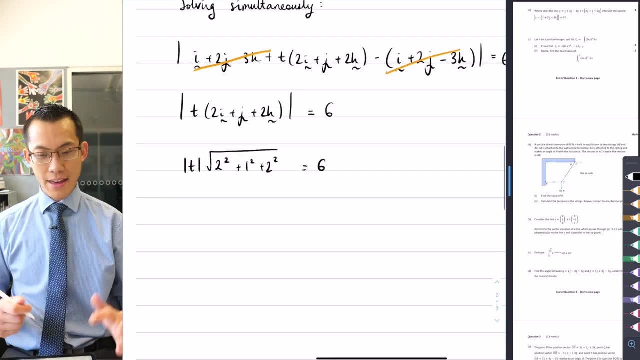 reading off my i and j and k coefficients. right, That's how far I'm moving in the x, the y and the z directions. That is equal to 6, and then I just need to do a bit of solving here. So 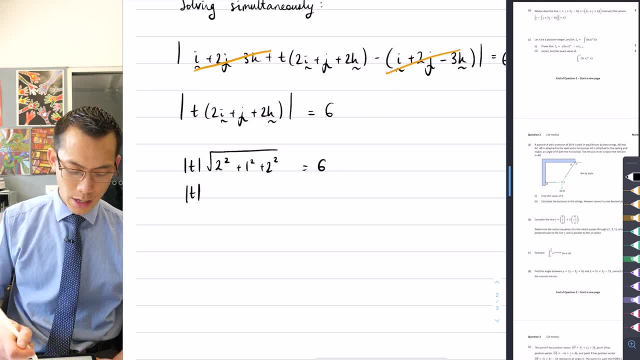 this is going to be absolute value of t. over here. This is 4 plus 1 plus 4, so that's 9.. So the square root of 9, last I checked- is 3.. That's equal to 6.. So now I'm getting the absolute value of t equals divide 3 by 3,. 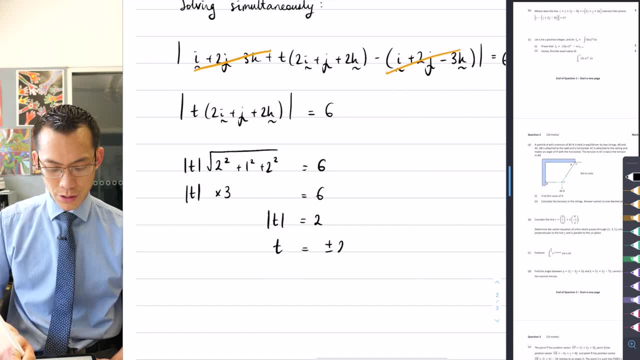 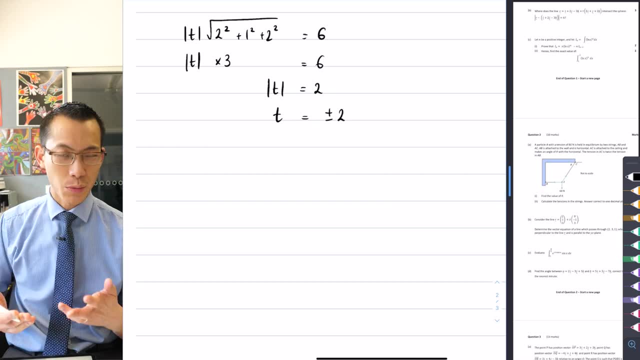 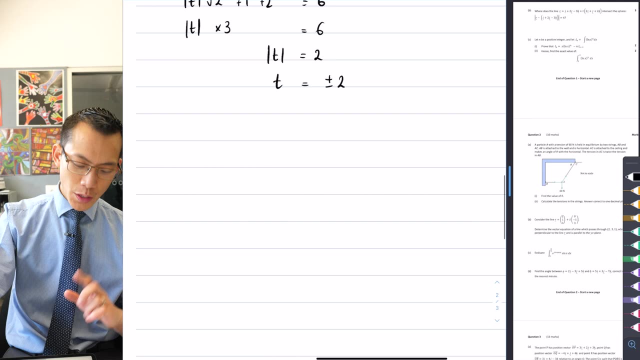 that gives me 2.. So t can be plus or minus 2.. So what I need to do is take these two parameters and pop them back into the line equation, because that's where t belongs, right, And that should give me two coordinates, two points on the line that intersect with the sphere. So substituting: 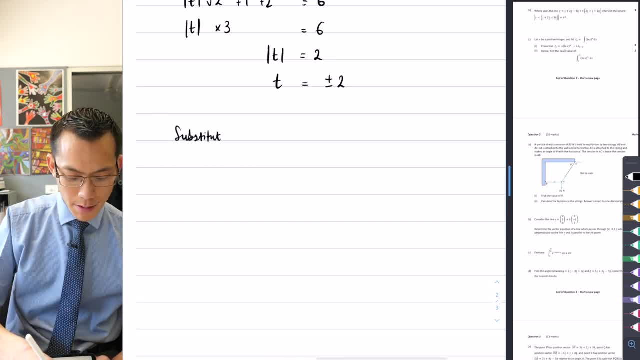 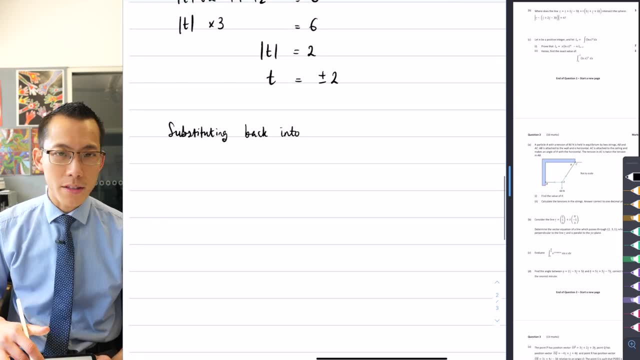 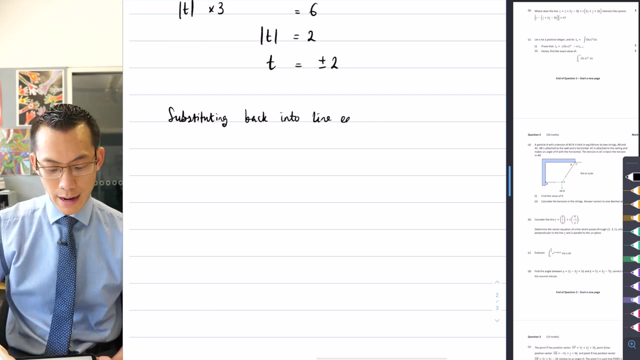 back into the line. equation- and I think it's really important Whenever you're working- takes a sort of left or a right turn. use words to make clear why the equations, or why one equation sort of gives way to another one. So substituting back into line. 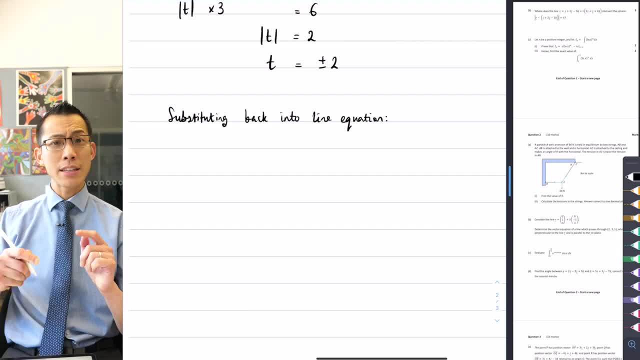 equation, because that's the only one that has t's in it. Let's do t equals 2.. So t equals 2 is going to give me a particular point. I'm going to call it point 1. And when I substitute it in, 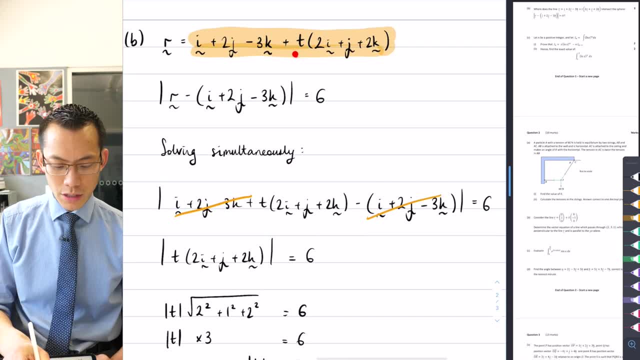 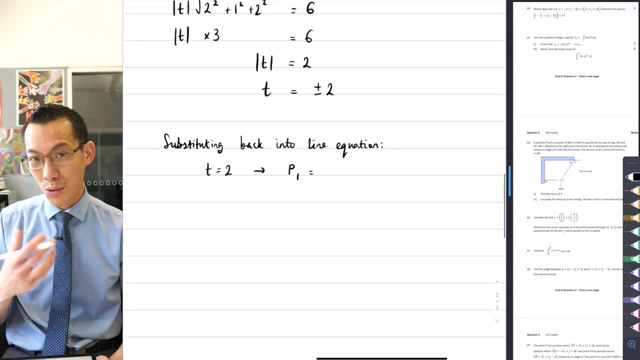 here is the line equation, right here. So the t equals 2 is going to go right there. Now, just to be lazy for myself, I'm just going to write this in column form, because then I just don't have to write all the i's and j's and k's And mathematicians famously lazy, right. So here comes. 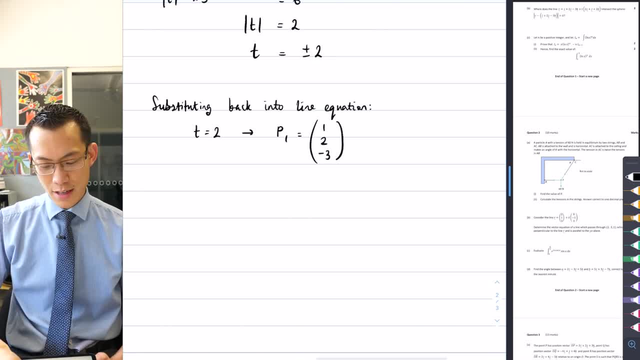 the column. It's 1, 2, negative 3.. There's my position vector, And then I'm going to add two. lots of you know. there's the parameter that I've substituted in: 2, 1, 2.. There we go, That's. 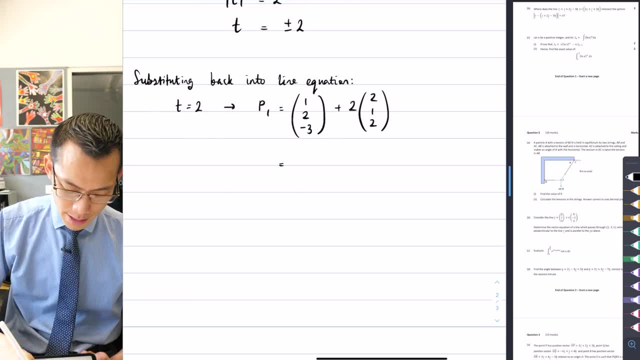 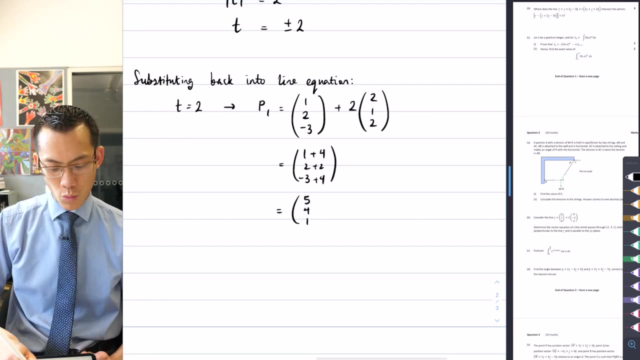 the direction vector. So when I have a look at that, let's see here. I'm going to compare my components here. So that's 1 plus 4 on the top, 2 plus 2 in the middle and negative 3 plus 4 on the bottom. So that's giving me 5, 4, and then 1. 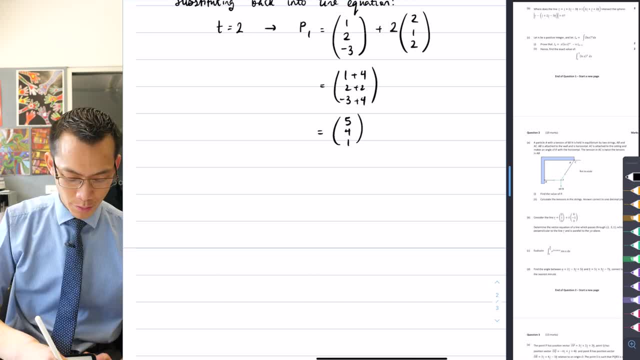 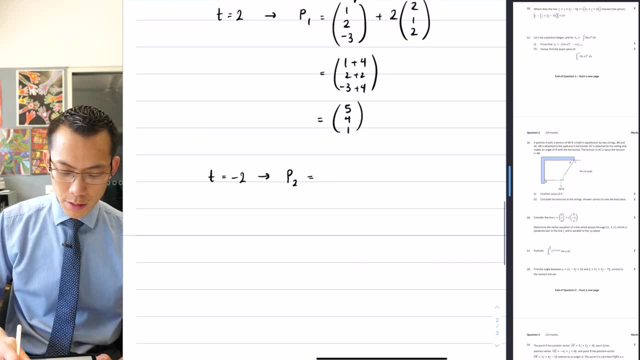 by the looks of things, Done that for the first parameter, Let's do it for the second, So here comes negative 2.. That's going to give me a secondary point And in fact it's going to look much like this first piece of working here, if I can copy and paste it properly, this first piece. 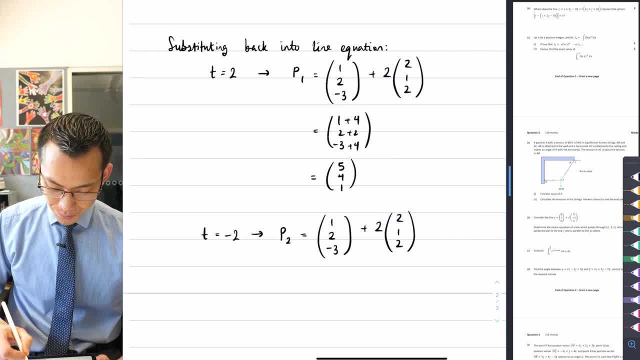 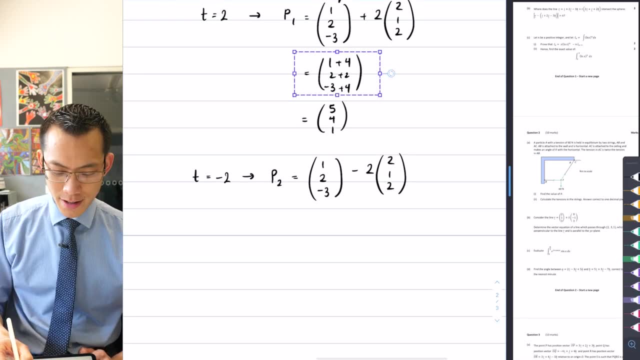 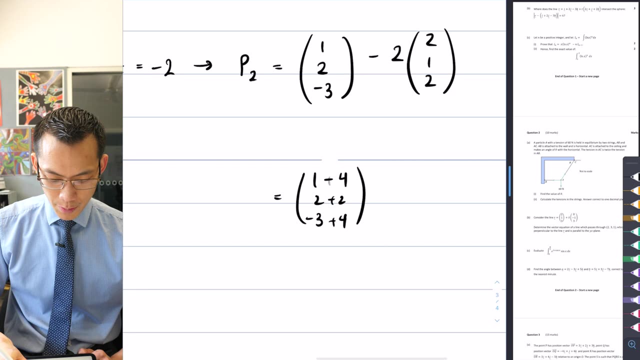 of working here, with just this one subtle difference, which is that minus sign right T equals negative 2. Which means I can be even lazier. Don't mathematicians love sort of saving the work? Everything here is going to start out the same, but I'm going to be subtracting this. 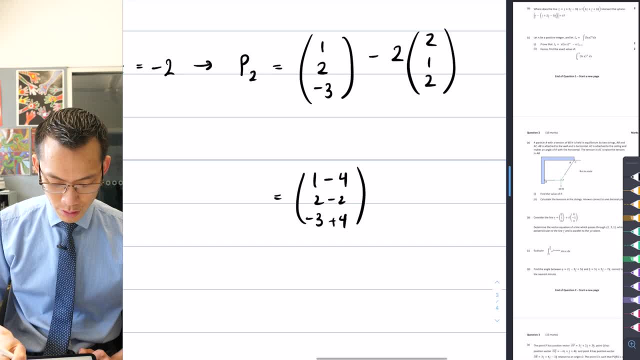 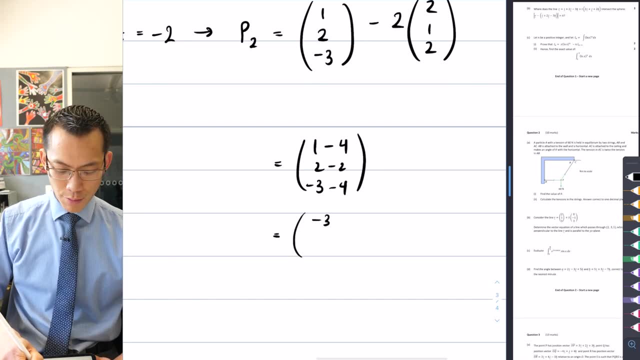 secondary vector here. So it'll be 1 minus 4,, 2 minus 2, and then minus 3 minus 4.. So I can just do the arithmetic on this. Let's see That's going to be a negative 3.. You get a 0 and a negative 7.. So that's p2 and that was p1 up there. So that's my, you know, the second vector here, And then I'm going to do the arithmetic on that. So that's going to be, you know, a negative 2 plus 3.. And then I'll 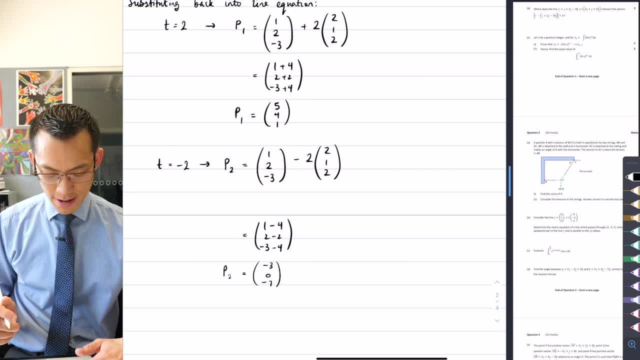 get a negative 7.. So that's p2 and that was p1 up there. So that's the only way I'm going to get the P1 up there. So I'm pretty much done. I should tie this up neatly in a bow, because I was. 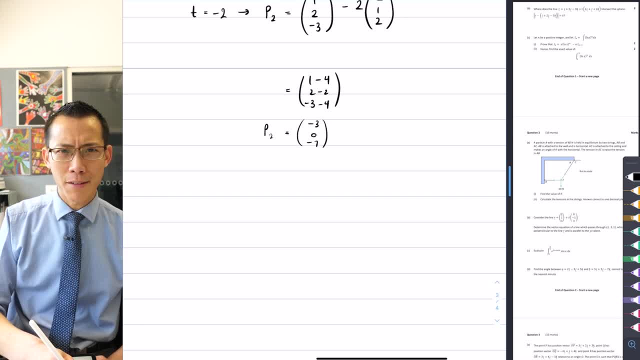 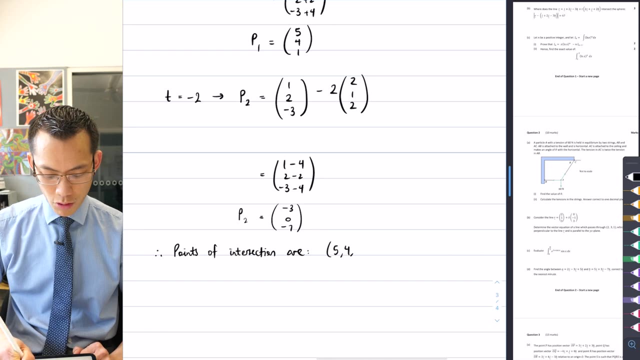 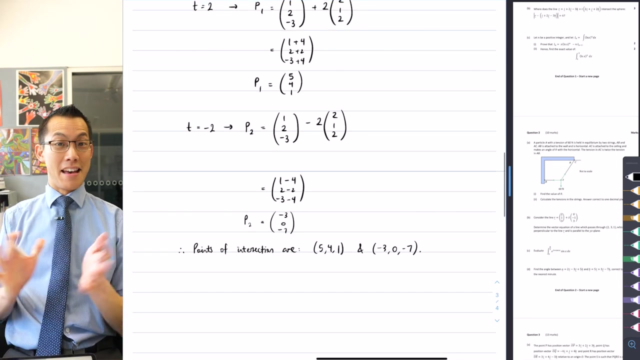 asked for points of intersection, not vectors. that point at points of intersection. so therefore I'm going to say the points of intersection are and let's just write them in coordinate form: are we get 5,, 4, 1? the first time wasn't it 5, 4, 1 and negative 3, 0, negative 7.. 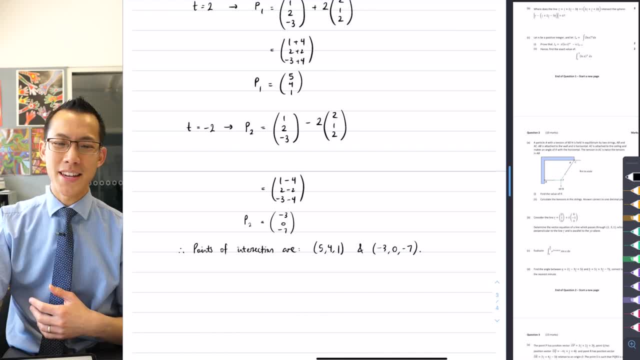 Happy times. Okay, so we have just found the points of intersection between that line and the sphere. The next question is going to be about integration.